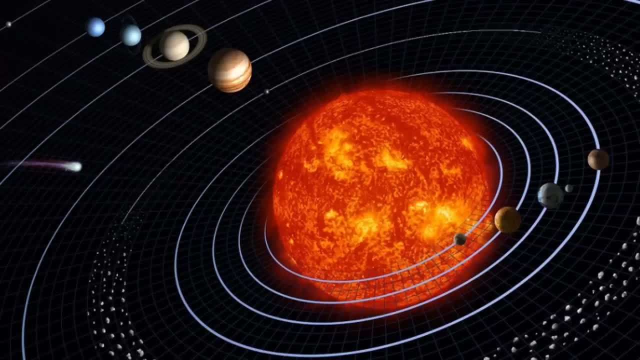 around and around and around the sun Isn't that cool. They just go around and around. It's really awesome. The sun is in the center and the planets just, oh, they go around. That's called orbiting. And you see, these lines, these circle lines. that's showing the pathway of these planets going. 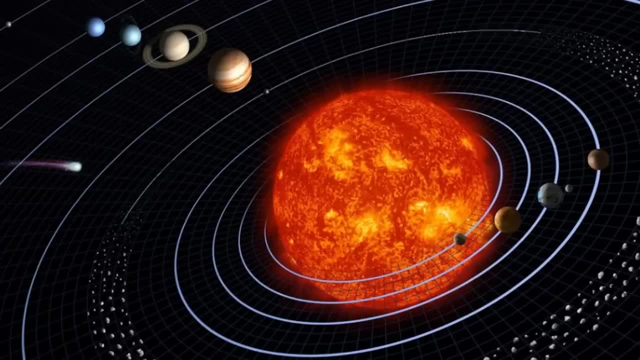 around the sun. I wonder if the sun ever gets annoyed with that. It's just like: hey, you know, leave me alone. You planets have been circling around me over and, over and over again and I'm sick of it. Get out of the way. I'm sick of it. I'm sick of seeing you go around me. I'm the center. 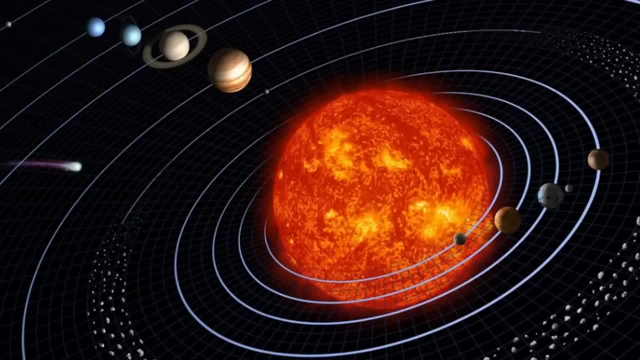 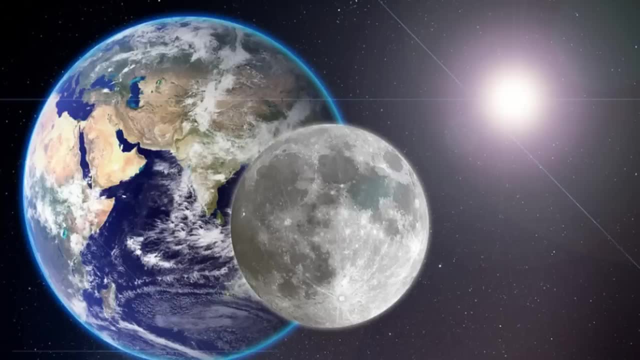 of the solar system, but please leave me alone. Well, the earth has something orbiting around it, just like the planets orbit around the sun, The moon orbits around the earth and the moon has been going around and around the earth, just like the planets go around and around the sun. All right, So what is a solar eclipse? 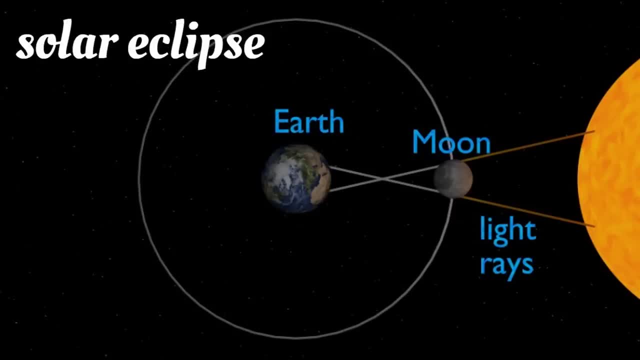 A solar eclipse is when the sun is in the center of our solar system, When the earth, moon and sun align And the light rays from the sun are blocked because the moon is in the way and the shadow of the moon hits the earth, making it look dark and obscuring. 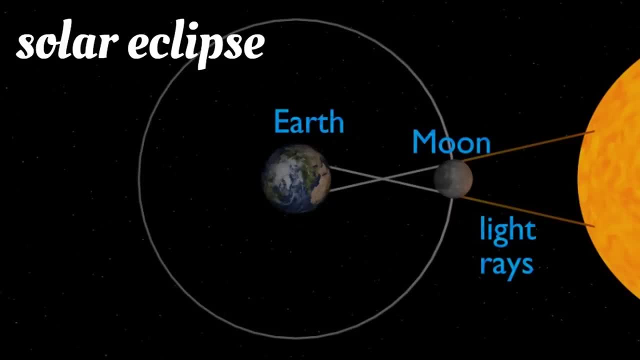 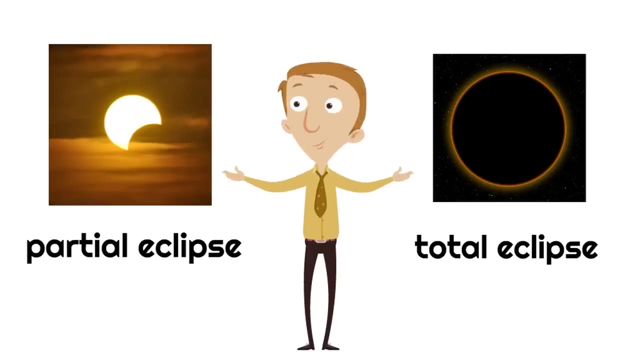 That means blocking, darkening the sun. How cool is that. They're aligned. It's really awesome and it's super rare, because it just doesn't happen that often. Now, there are two types Of solar eclipses. there's a partial eclipse, That's when part of the sun is blocked by the moon. 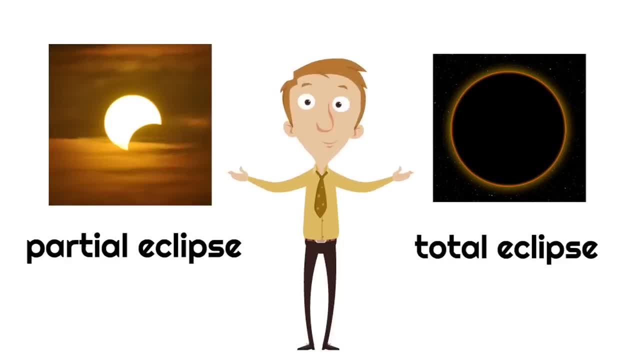 And then there's a total eclipse, where the entire sun is blocked. The total eclipse is the rarest of all, but a partial eclipse is really special too. If you ever get to see a solar eclipse, even if it's a partial eclipse, you're gonna want to, because 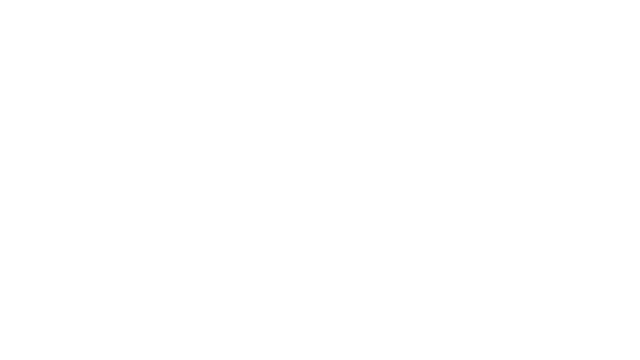 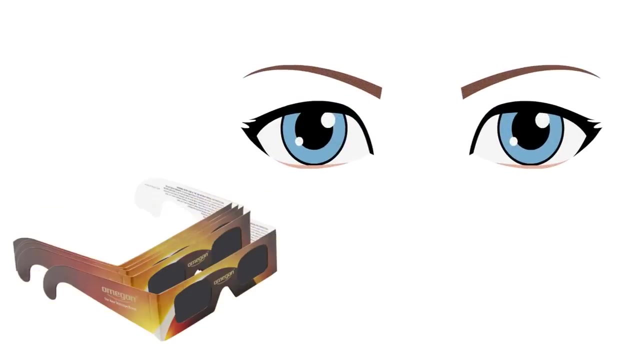 it's so cool. Just make sure you protect your eyes when you enjoy a solar eclipse. Make sure you're wearing special glasses that protect them from the sun, because it's never a good idea to look directly at the sun. The only time it's safe to take off your solar glasses is when an adult tells you you. 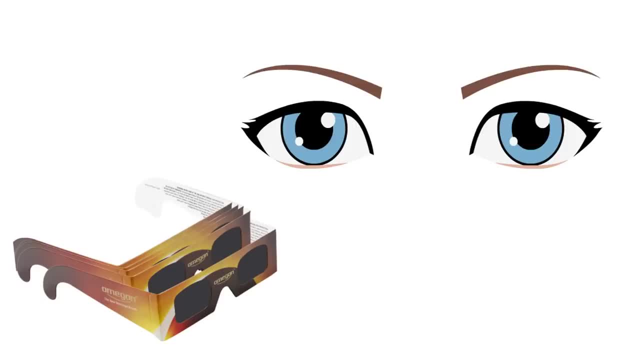 can when it reaches totality, which that's when it's completely blocked. That's if you're seeing a total eclipse. If it's a partial eclipse, you're gonna want to wear special glasses. You need to keep your solar glasses on the entire time. 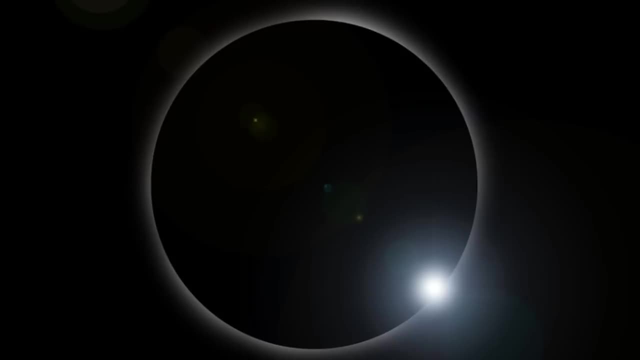 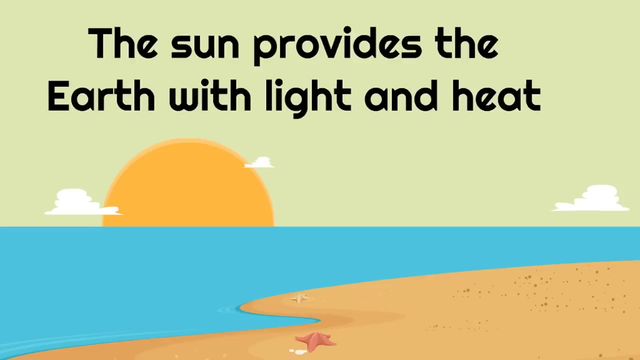 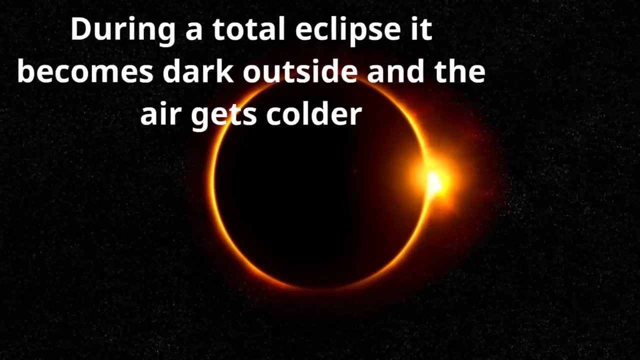 Now here's something really fascinating about a solar eclipse. The sun provides the Earth with light and heat. It's basically a burning ball of fire in the center of our solar system, Which means during a total eclipse it becomes dark outside and the air gets colder because- remember the 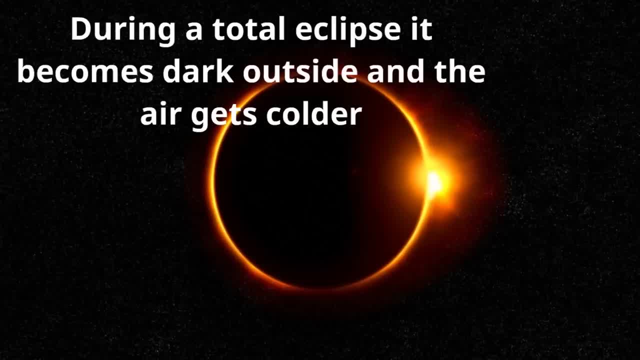 moon is blocking sunlight and is even blocking some of that heat. How awesome is that? How awesome is that Question for our guests- Why is that so cool? I don't know. Why is it so cool? Why is it so cool? 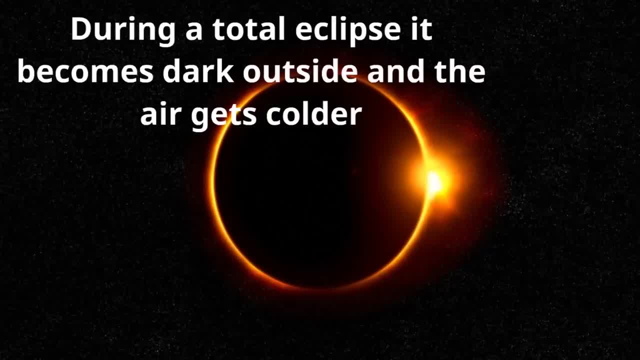 I don't know, Isn't it neat? Why is it dark outside and the air gets colder? Now this might sound silly, but it's absolutely true. They found that animals get confused during a total eclipse, which makes sense because all of a sudden, the sun� 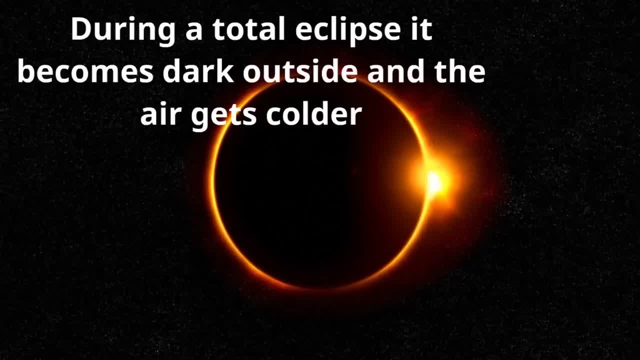 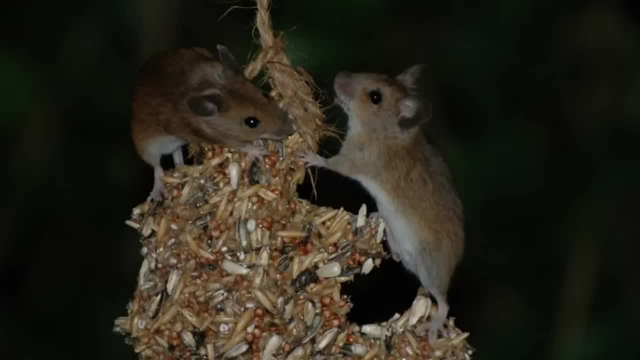 lives on the surface veterinally sudden. hey, you know what happened. who turned the lights down? who turned the lights? what's going on? these poor mice, they have no idea what's going on. they can't watch homeschool pop videos like you can. they don't know what's going on. they don't know what a solar eclipse is. they don't. 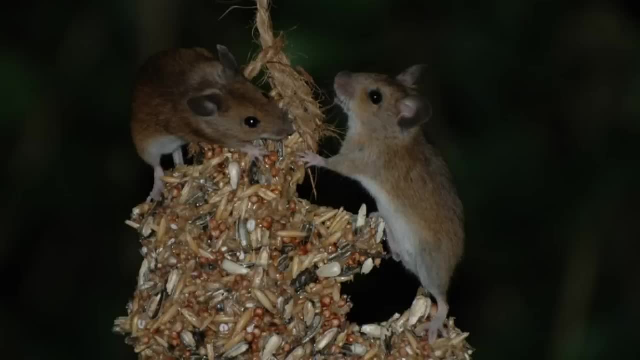 understand that the moon is covering the sun and is casting its shadow on the earth. they don't know, they're confused. but hold on, little mice, okay, it's okay. in about seven minutes a total eclipse is done and life will be normal. life will be normal again, it's okay. it's okay. i just don't.